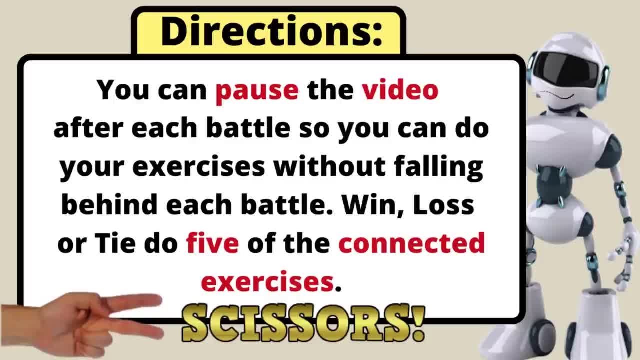 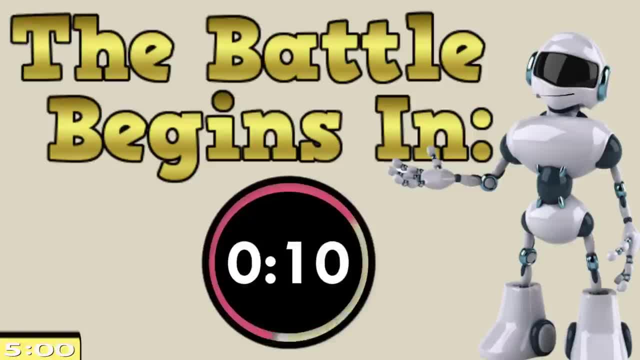 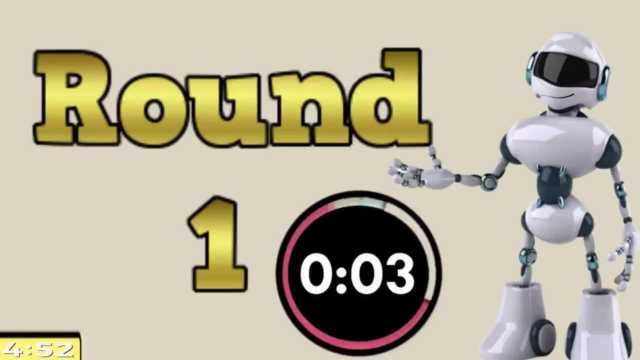 Let's see who wins. You can pause the video after each battle so you can do your exercises without falling behind each battle. Win, lose or tie. do five of the connected exercises. The battle begins in nine, eight, seven, six round one, four, three, two, one rock paper scissors: shoot. 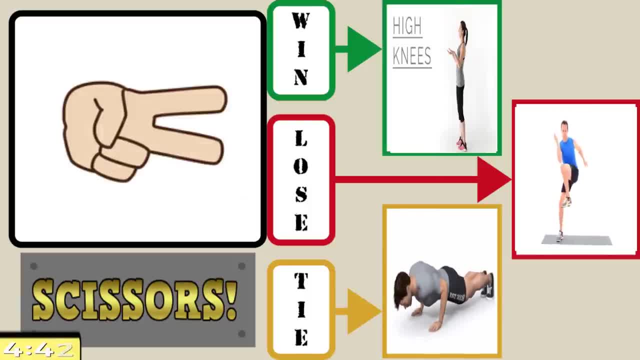 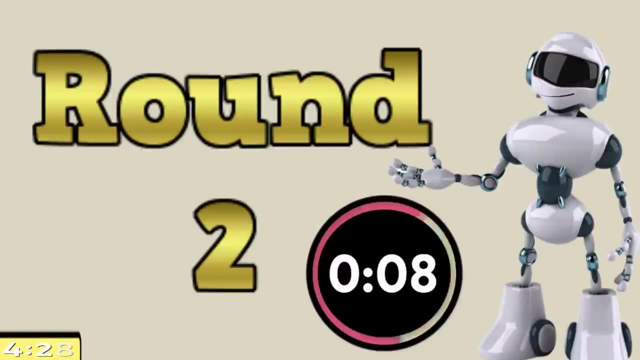 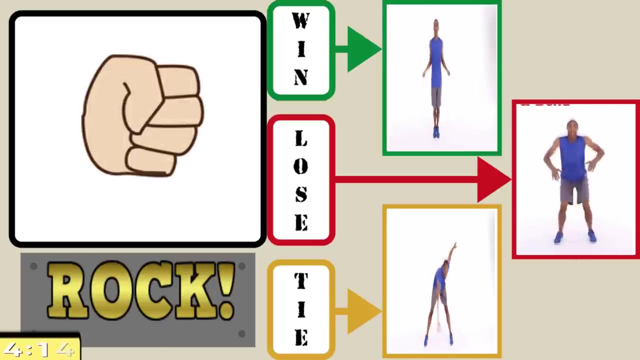 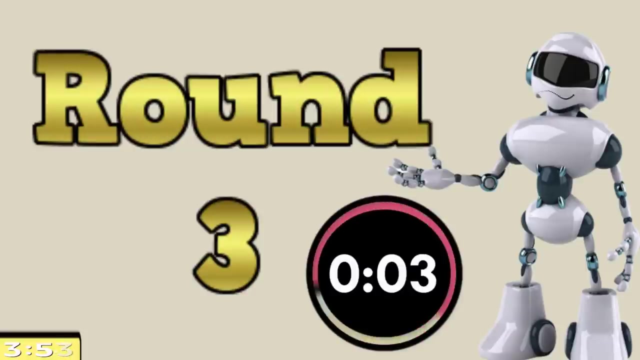 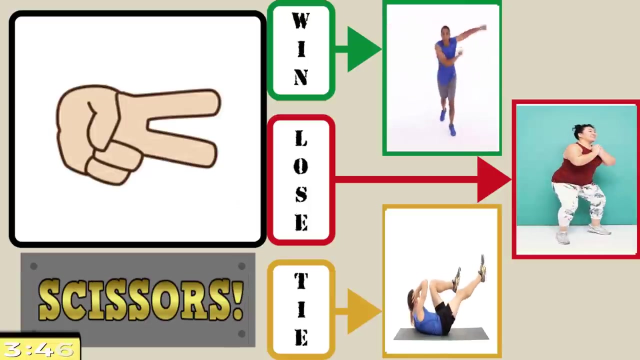 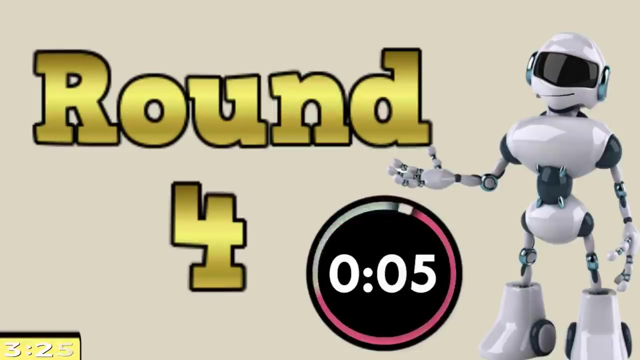 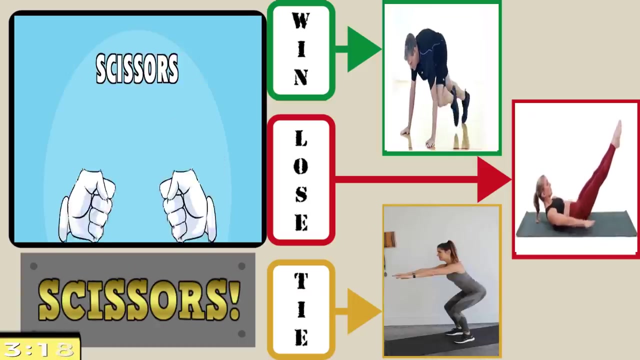 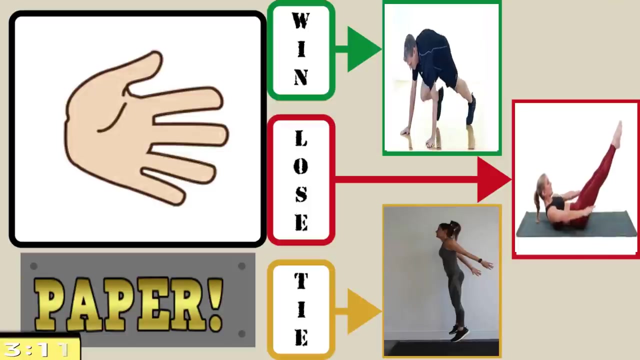 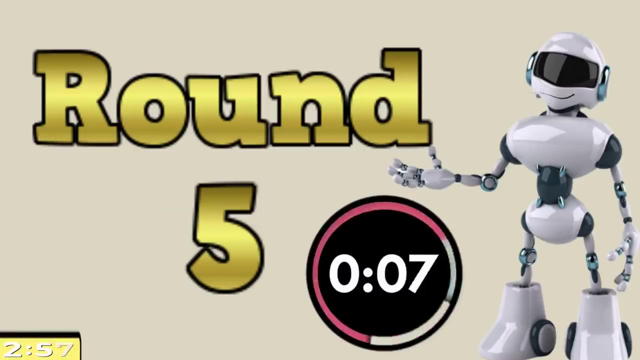 round two: nine, eight, seven, six, five, four, three, two one rock paper scissors shoot round three: nine, eight, seven, six, five, four, three, two. one rock paper scissors shoot round four. nine, eight, seven, six, five, four, three, two. one rock paper scissors shoot round four. nine, eight, seven, six, five, four, three, two one rock paper scissors shoot. 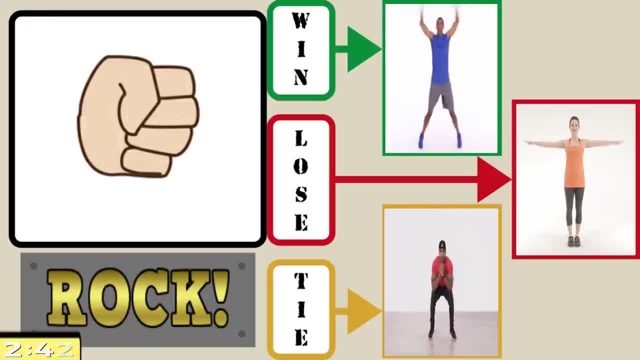 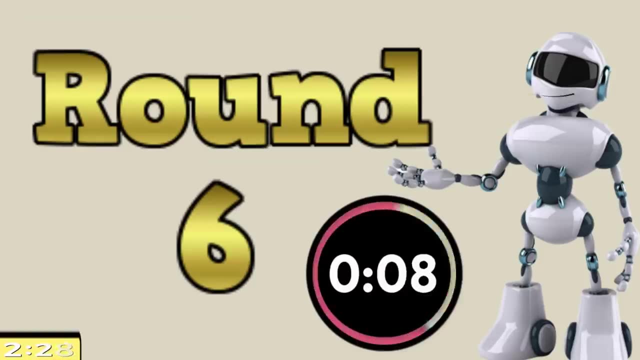 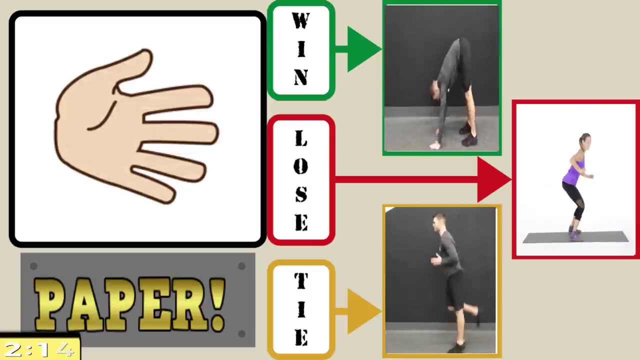 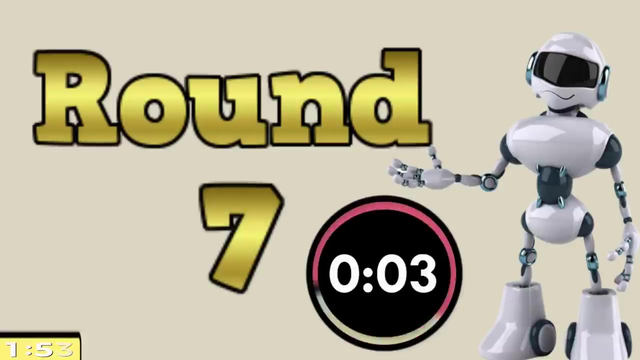 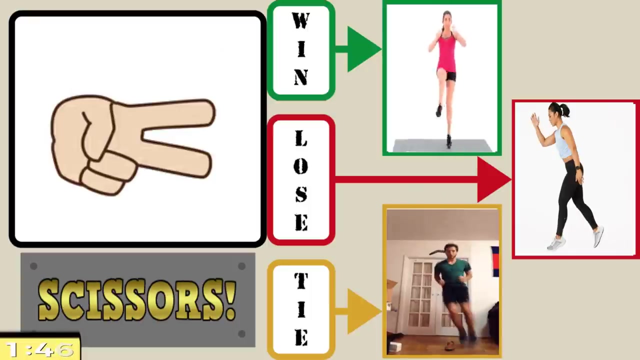 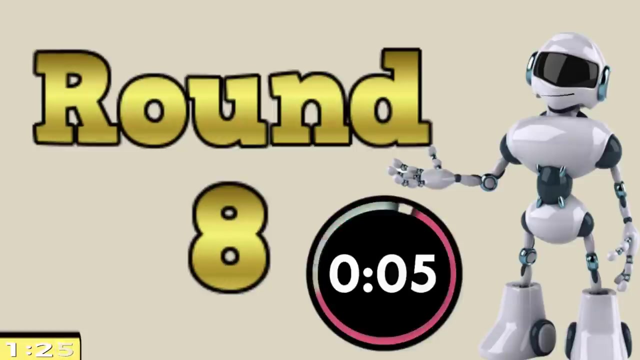 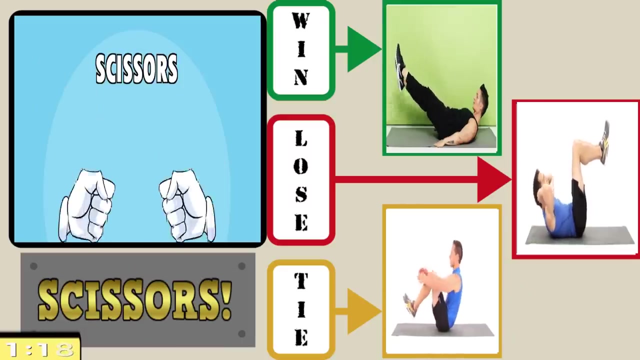 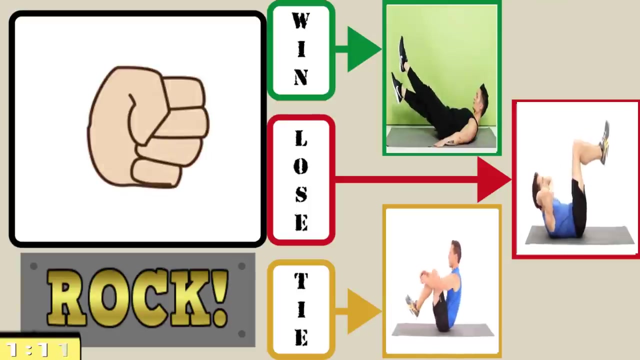 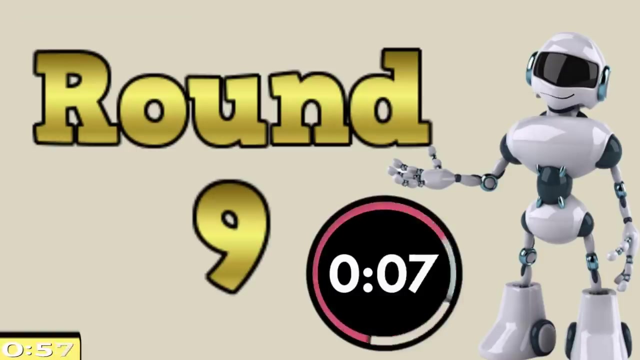 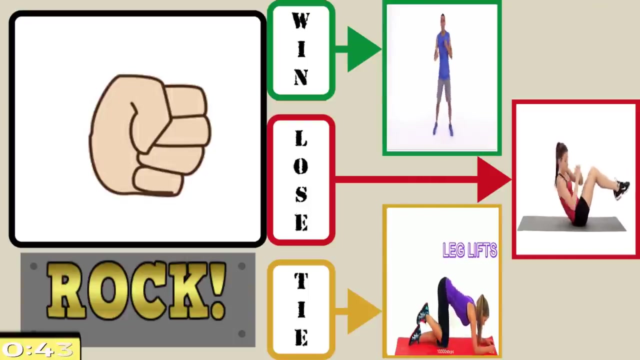 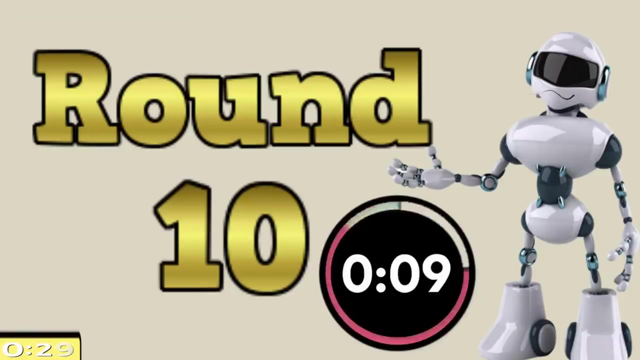 Round 6: Rock paper scissors shoot. Round 7: Rock paper scissors shoot. Round 8: Rock paper scissors shoot. Round 9: Rock paper scissors shoot. Round 10: 9,, 8,, 7,, 6,, 5,, 4,, 3,, 2, 1. 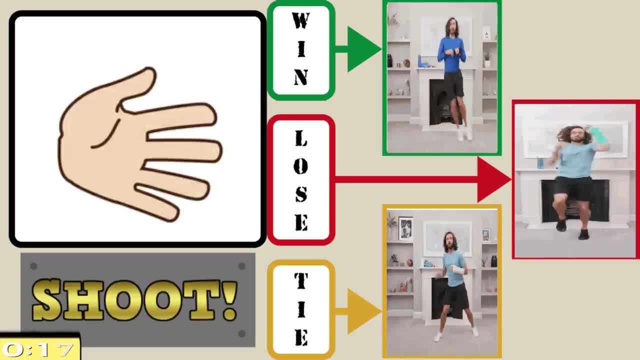 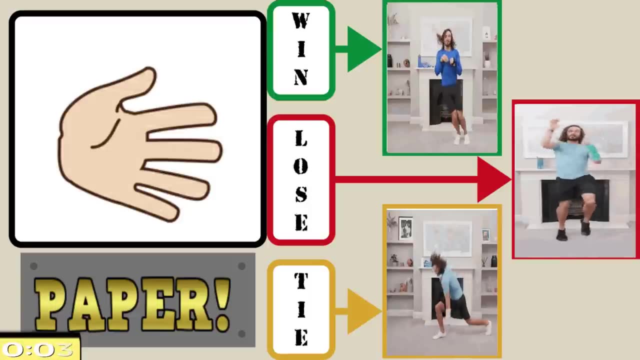 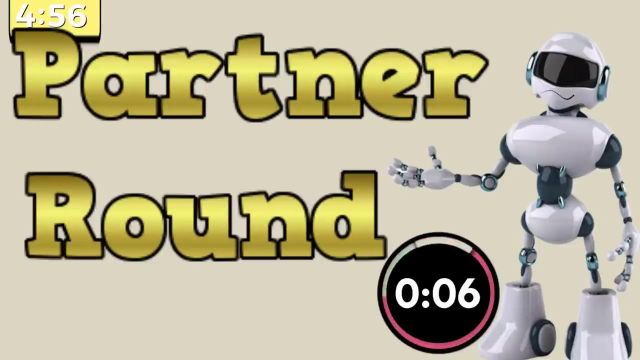 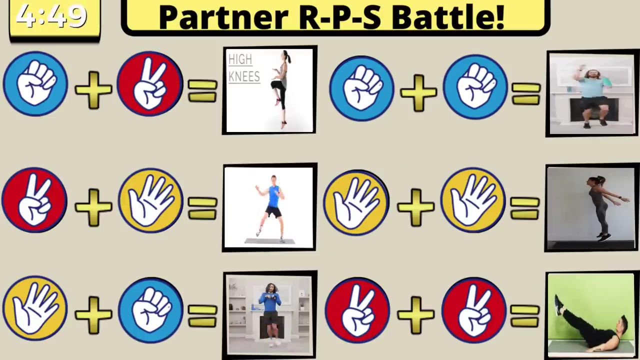 Rock paper scissors shoot- Round 11: 9,, 8,, 7,, 6,, 5,, 4,, 3,, 2, 1. Rock paper scissors shoot- Round 12. Rock paper scissors shoot. 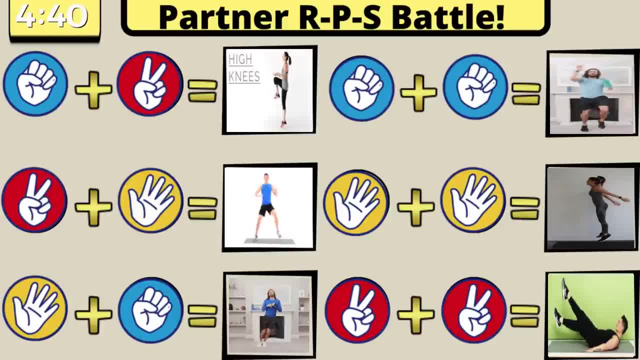 Round 13: Rock paper scissors shoot Round 14: Rock paper scissors shoot Round 15. Rock paper scissors shoot Round 16. Rock paper scissors shoot Round 17: Rock paper scissors shoot Round 18. 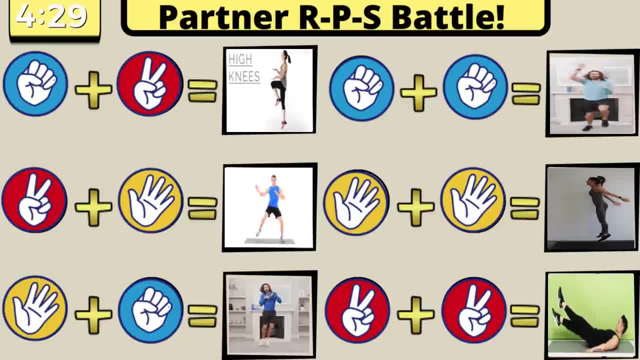 Rock paper scissors shoot Round 19. Rock paper scissors shoot Round 20. Rock paper scissors shoot Round 21. Rock paper scissors shoot Round 22. Rock paper scissors shoot Round 23. Rock paper scissors shoot. 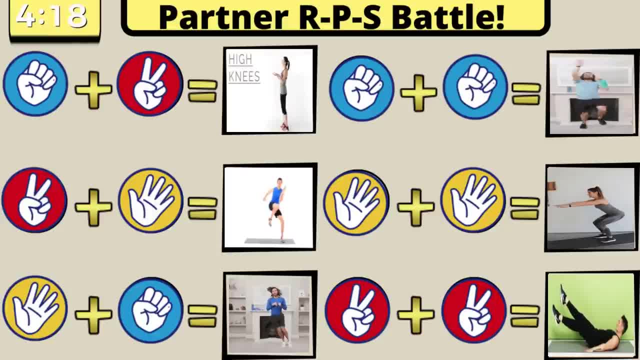 Round 24: Rock paper scissors: shoot Round 25. Rock paper scissors: shoot Round 26. Rock paper scissors: shoot Round 27. Rock paper scissors: shoot Round 28. Rock paper scissors- shoot Round 29. 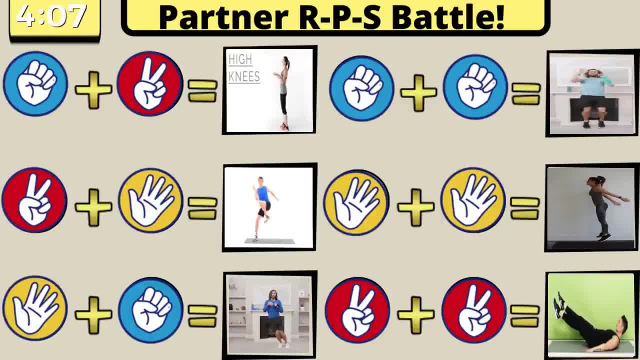 Rock paper scissors: shoot Round 30. Rock paper scissors: shoot Round 31. Rock paper scissors: shoot Round 32. Rock paper scissors: shoot Round 33. Rock paper scissors: shoot Round 34. Rock paper scissors shoot. 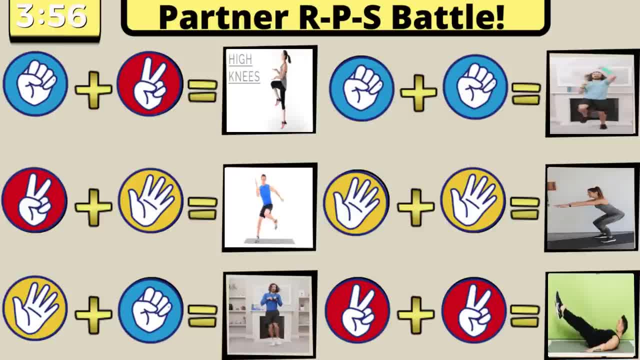 Round 35: Rock paper scissors: shoot Round 36. Rock paper scissors: shoot Round 37. Rock paper scissors: shoot Round 38. Rock paper scissors: shoot Round 39. Rock paper scissors: shoot Round 40. 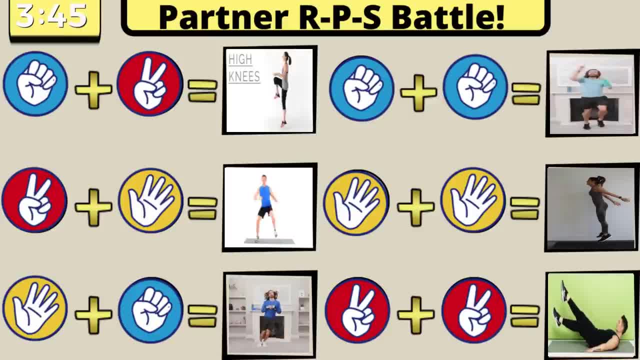 Rock paper scissors: shoot Round 41. Rock paper scissors: shoot Round 42. Rock paper scissors: shoot Round 43. Rock paper scissors: shoot Round 44. Rock paper scissors: shoot Round 45. Rock paper scissors shoot. 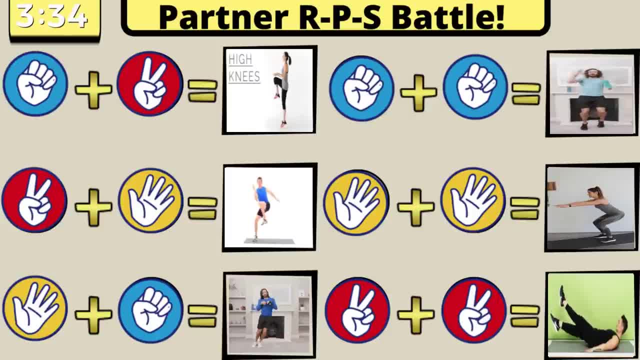 Round 46: Rock paper scissors: shoot Round 47. Rock paper scissors: shoot Round 48. Rock paper scissors: shoot Round 49. Rock paper scissors: shoot Round 50. Rock paper scissors: shoot Round 51. 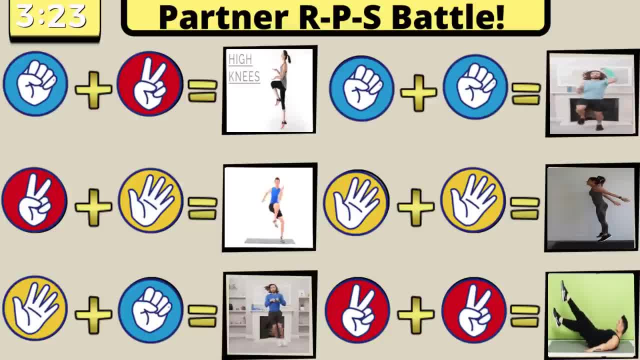 Rock paper scissors: shoot Round 52. Rock paper scissors: shoot Round 53. Rock paper scissors: shoot Round 54. Rock paper scissors: shoot Round 56. Rock paper scissors: shoot Round 57. Rock paper scissors shoot. 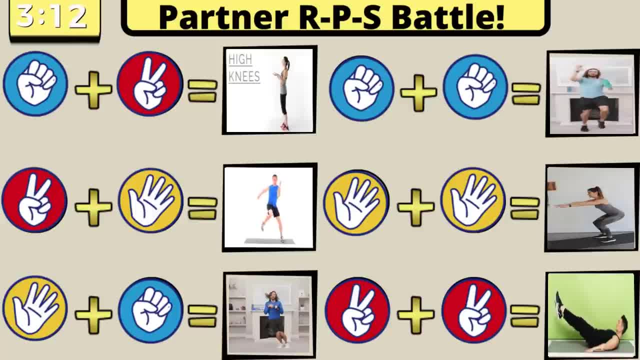 Round 58: Rock paper scissors: shoot Round 59. Rock paper scissors: shoot Round 60. Rock paper scissors: shoot Round 61. Rock paper scissors: shoot Round 62. Rock paper scissors: shoot Round 63. 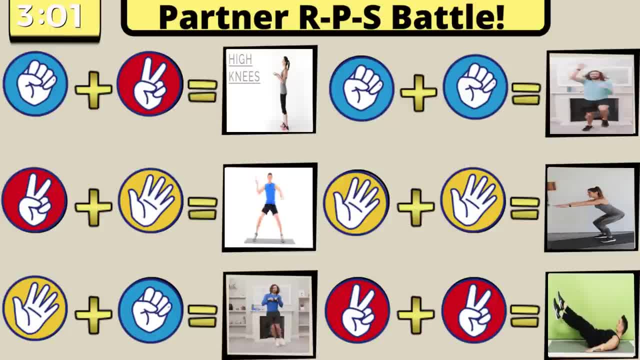 Rock paper scissors: shoot Round 64. Rock paper scissors: shoot Round 65. Rock paper scissors: shoot Round 66. Rock paper scissors: shoot Round 67. Rock paper scissors: shoot Round 68. Rock paper scissors shoot. 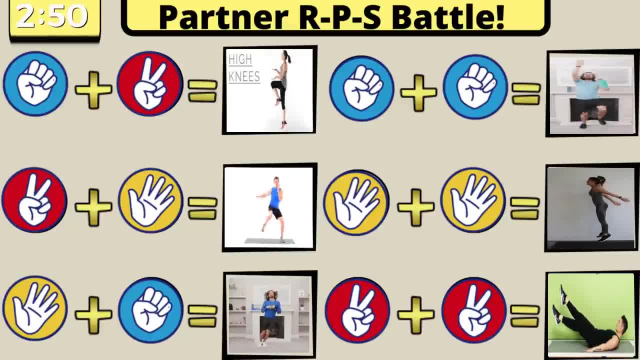 Round 69: Rock paper scissors: shoot Round 61. Rock paper scissors: shoot Round 62. Rock paper scissors: shoot Round 63. Rock paper scissors: shoot Round 67. Rock paper scissors: shoot Round 68. 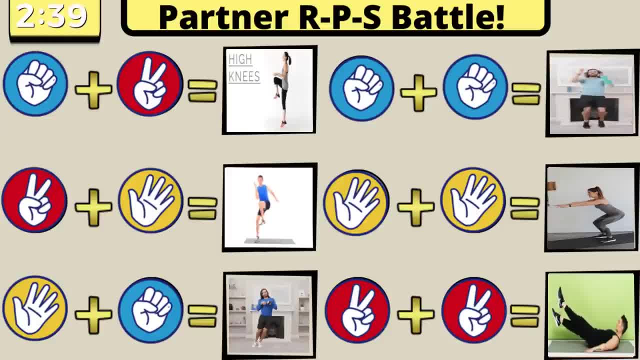 Rock paper scissors: shoot Round 69. Rock paper scissors: shoot Round 69. Rock paper scissors: shoot Round 70. Rock paper scissors: shoot Round 71. Rock paper scissors: shoot Round 72. Rock paper scissors shoot. 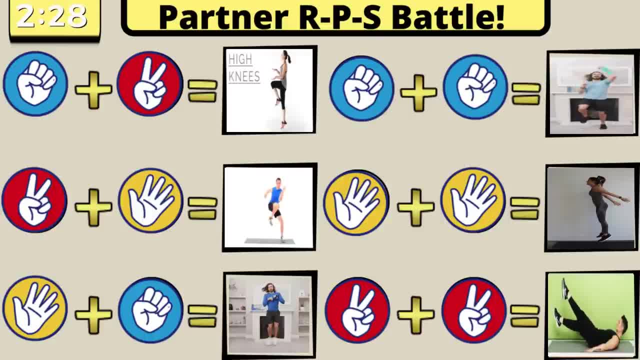 Round 73: Rock paper scissors: shoot Round 74. Rock paper scissors: shoot Round 75. Rock paper scissors: shoot Round 76. Rock paper scissors: shoot Round 76. Rock paper scissors: shoot Round 77. 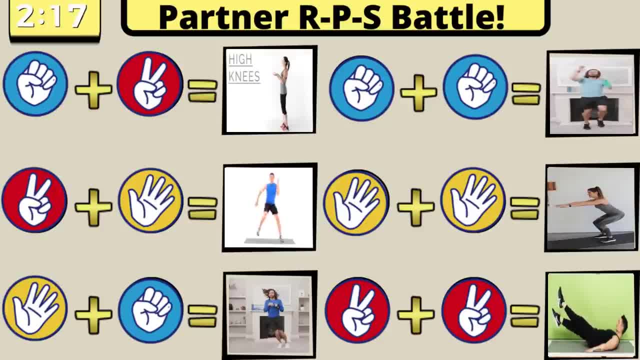 Rock paper scissors: shoot Round 78. Rock paper scissors: shoot Round 79. Rock paper scissors: shoot Round 80. Rock paper scissors: shoot Round 91. Rock paper scissors: shoot Round 92. Rock paper scissors shoot. 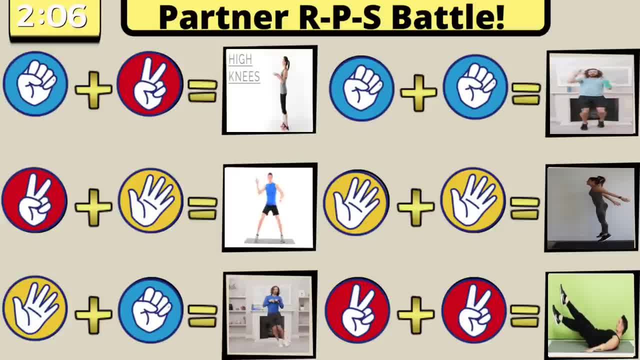 Round 93 Rock paper scissors. shoot Round 93 Rock paper scissors. shoot Round 94 Rock paper scissors. shoot Round 94 Rock paper scissors. shoot Round 95 Rock paper scissors. shoot Round 96. 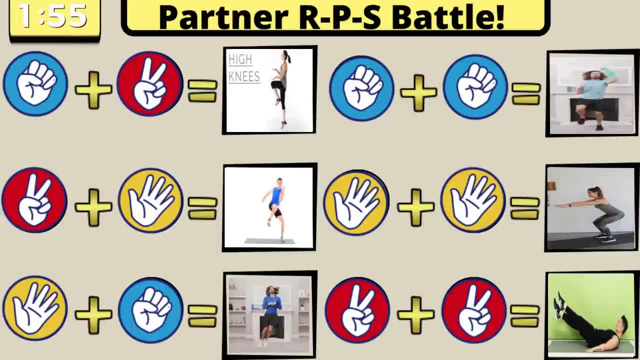 Rock paper scissors: shoot Round 97. Rock paper scissors: shoot Round 98. Rock paper scissors: shoot Round 99. Rock paper scissors: shoot Round 100. Rock paper scissors: shoot Round 100. Rock paper scissors shoot. 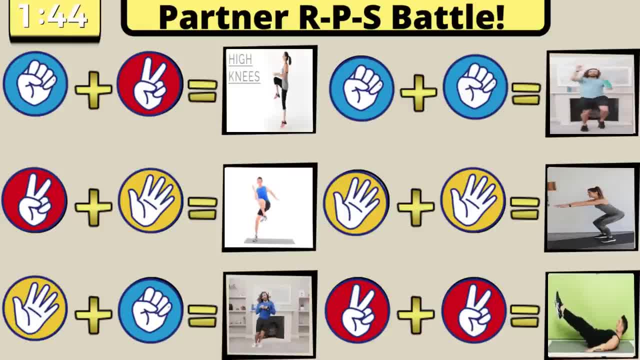 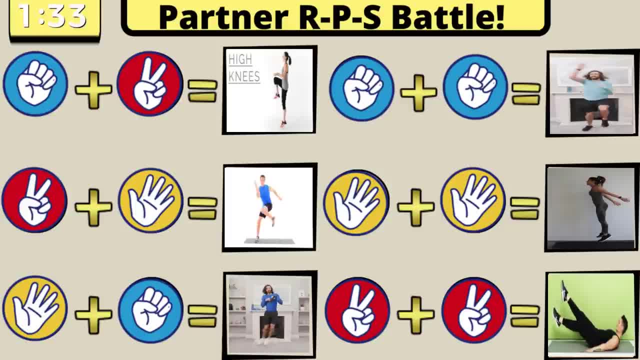 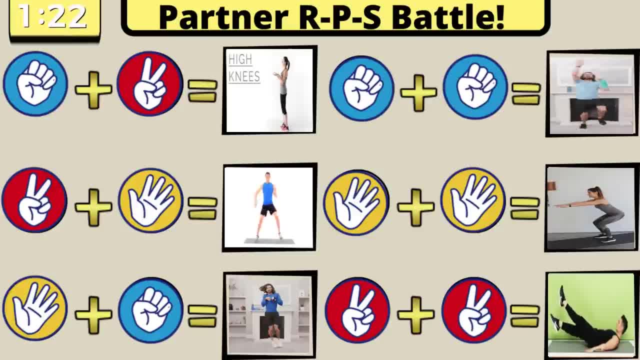 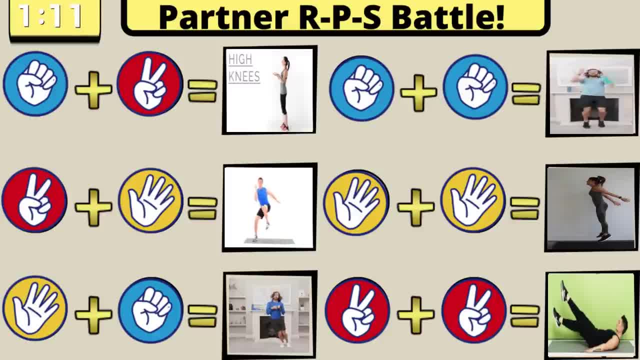 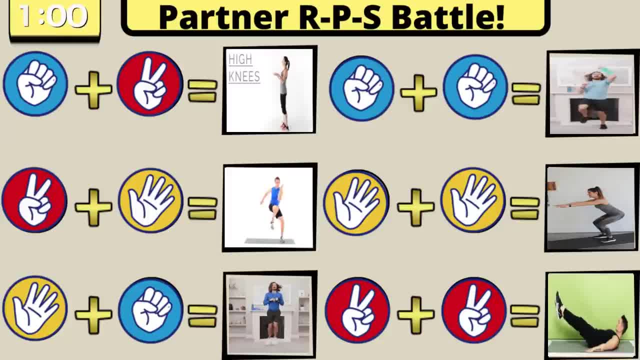 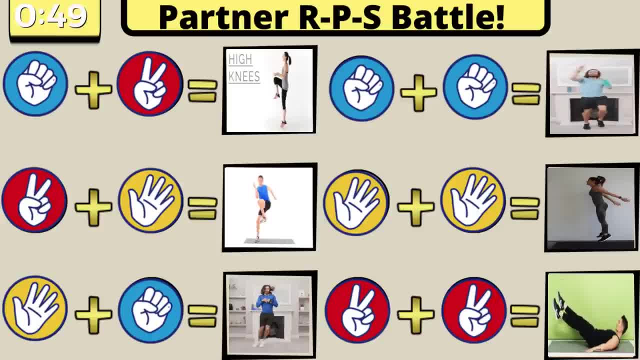 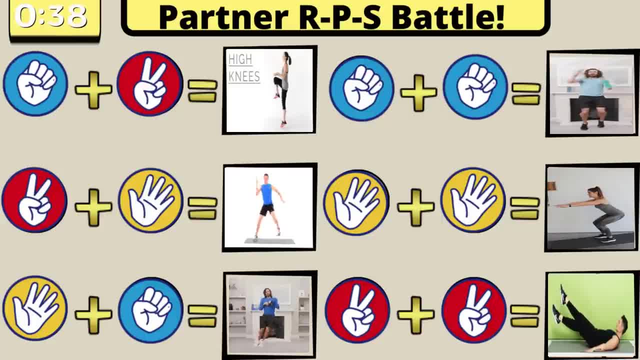